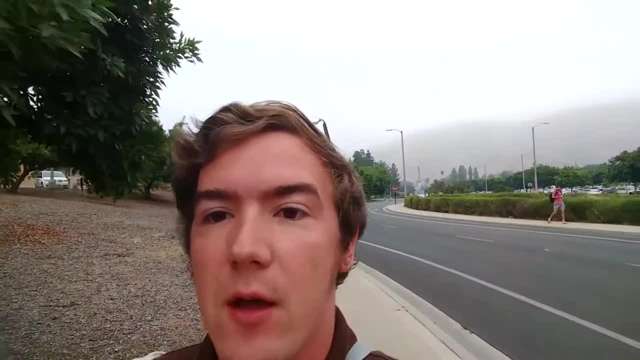 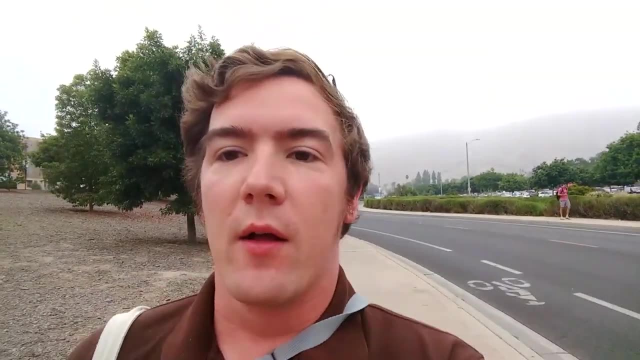 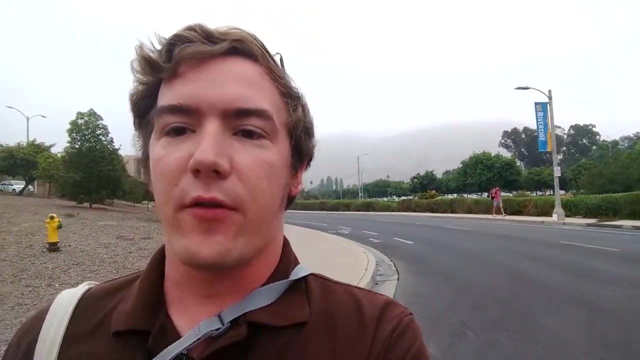 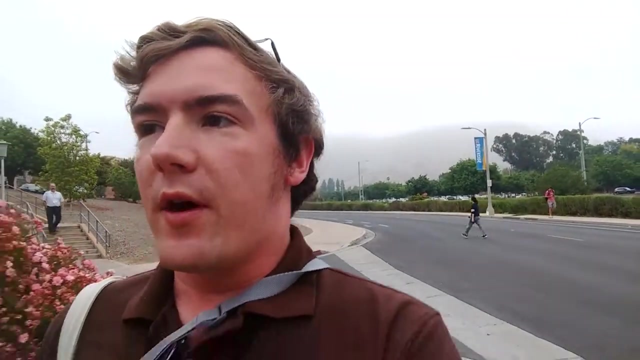 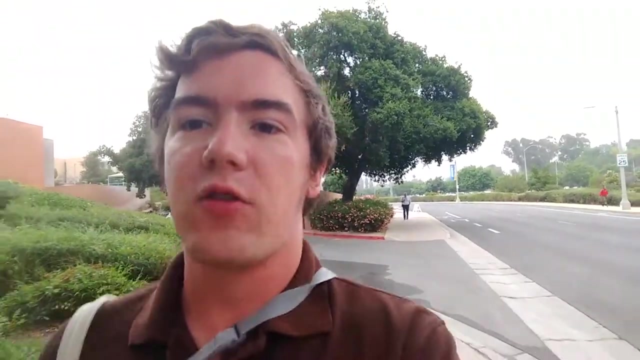 So rather big group. Even though it is the North America Paleontological Convention, we have a lot of people internationally as well, which is fantastic, And also the talks aren't just on North American fossils- There are fossils from all over the place. But it's a really good time to learn what other people are doing, to network with other people, get into contact so you can do collaborations with people and also just catch up with friends. 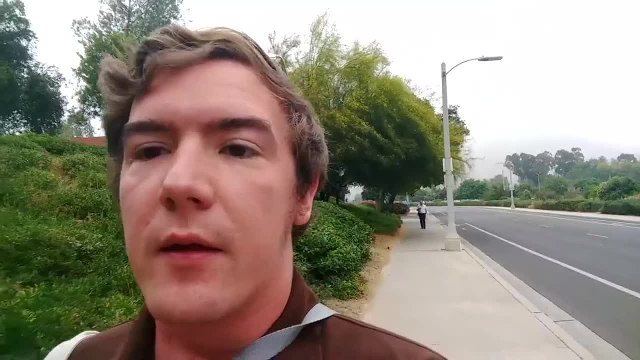 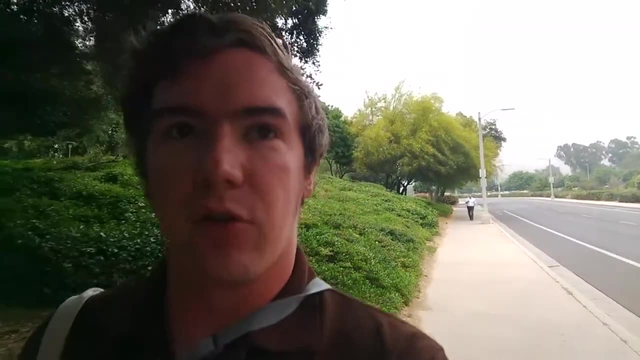 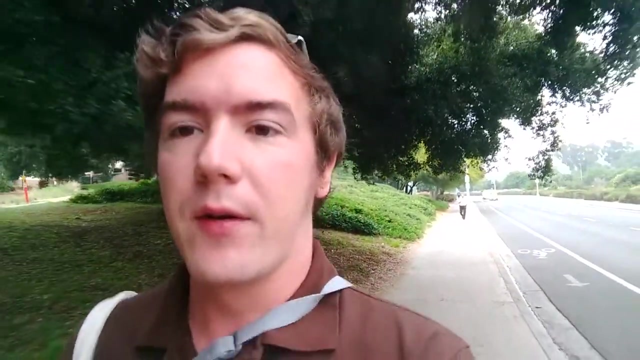 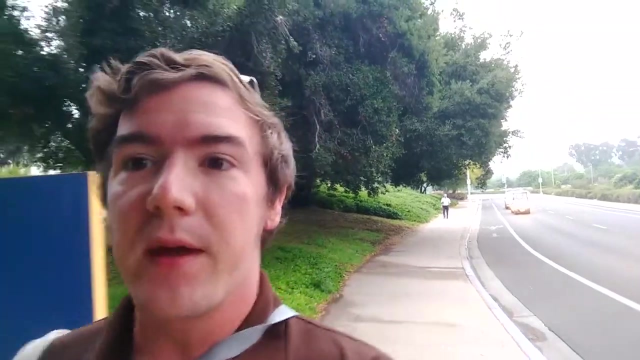 And people that you know in the field as well. So this is actually day three of the conference and I've talked a lot about people giving talks and lectures, which I think is you know what a lot of people think of, at least in paleontology. well, at least in any academic field, when you talk about conferences you're giving a presentation, a PowerPoint, usually about 15 minutes, in front of your peers. 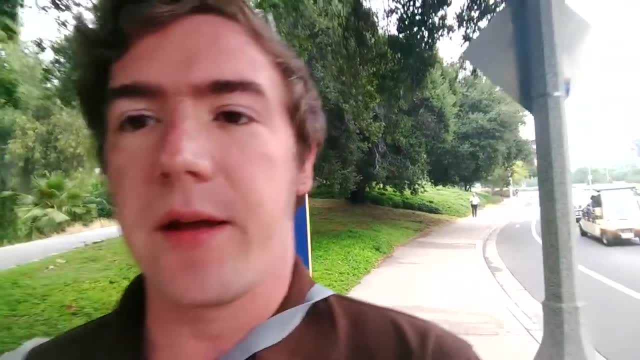 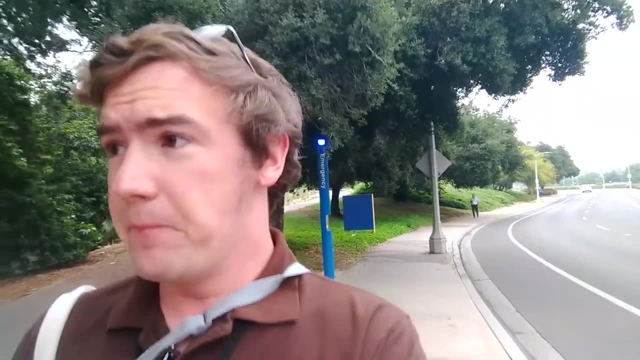 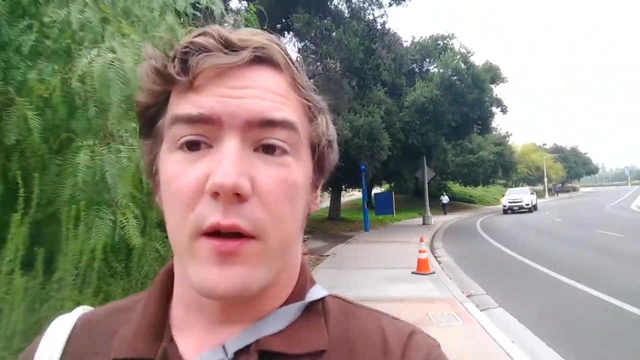 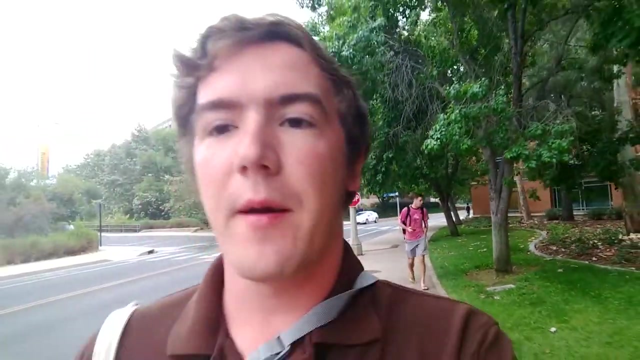 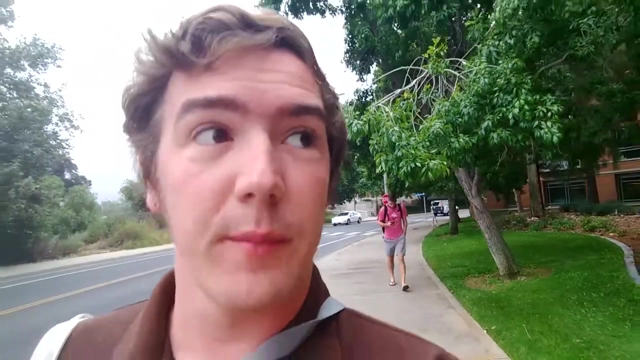 But there are also things like posters. Posters can convey a lot of information graphically, And then also people who are presenting posters can also help explain and answer questions during the poster sessions. A lot of times at conferences like this one or Geological Society of America, you'll have things like field trips that are a possibility so you can learn a little bit about geology and paleontology of the area. 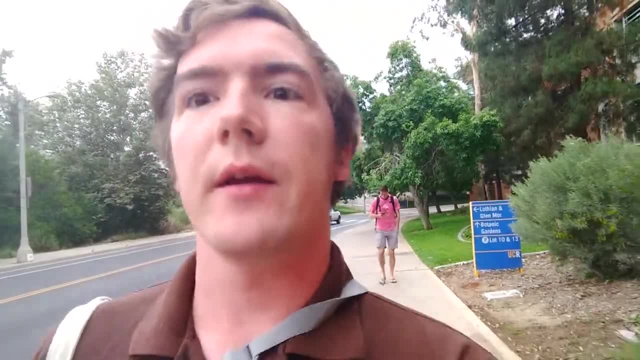 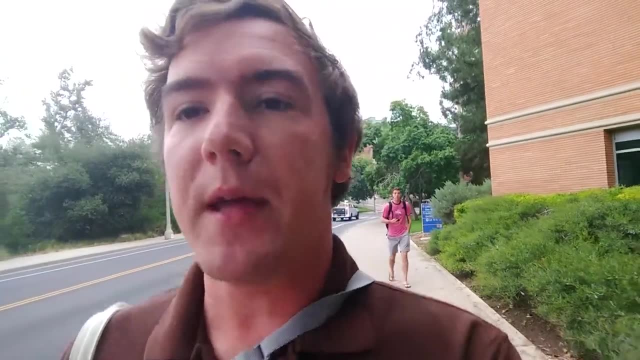 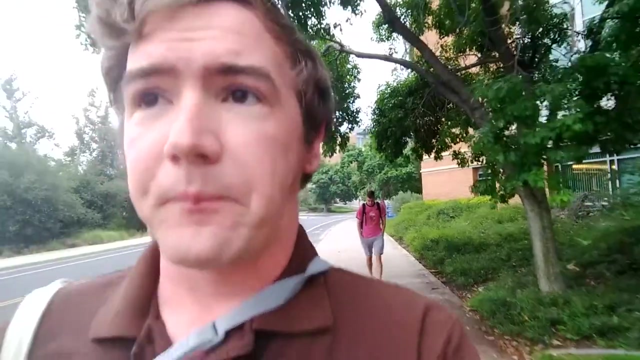 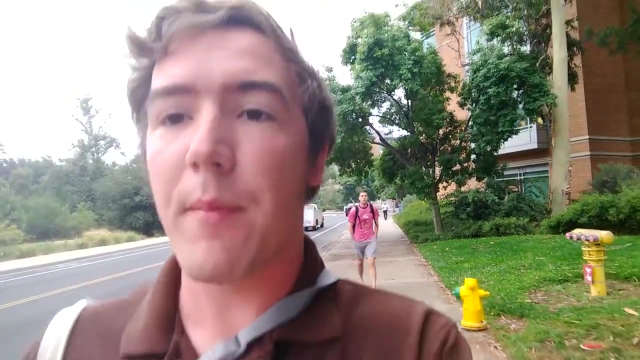 And there's also workshops, So yesterday I attended one on the Paleobiology Database, the PBDB, which is a free resource which we can include down in the link below. It contains a lot of data on published fossils and where they would have been geographically. 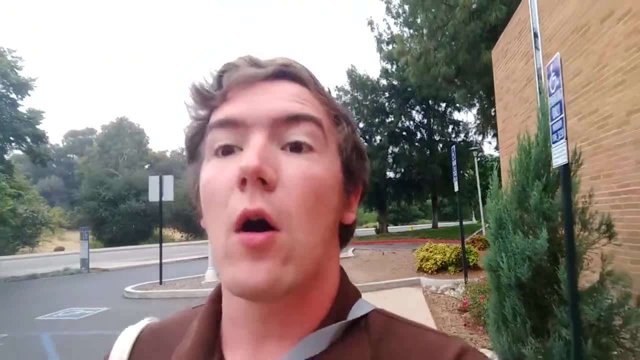 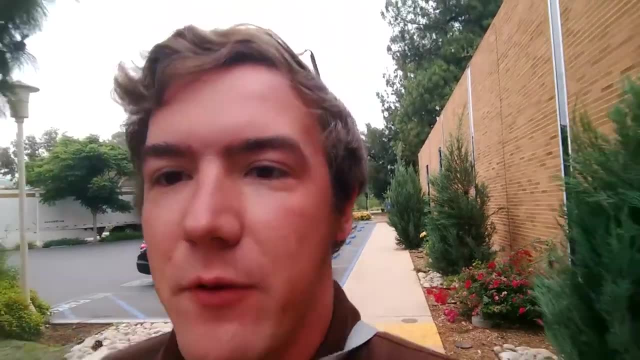 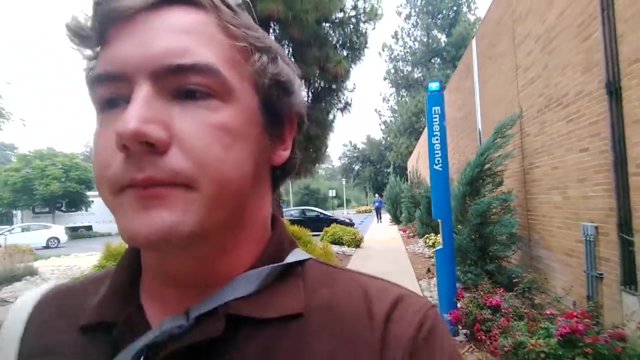 And so it's a lot of fun, and so you can see where all these things were living together spatially. so we're just gonna continue on down the main event. I'm staying right here on campus. a lot of the other presenters are staying here on campus as well, which so 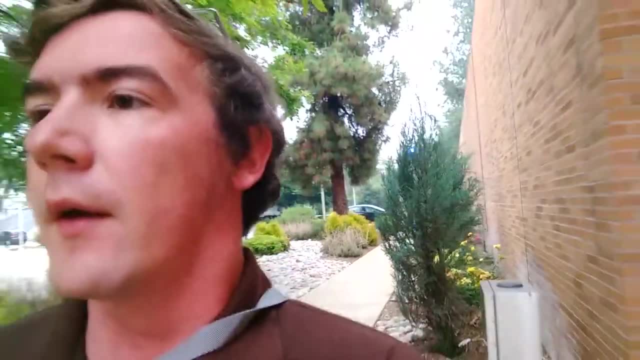 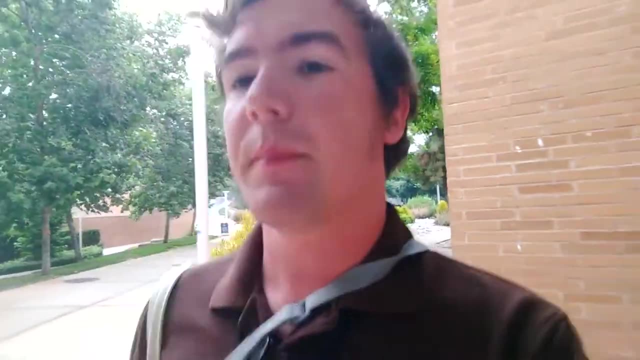 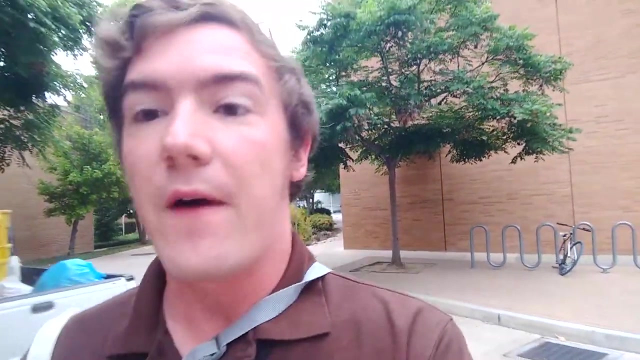 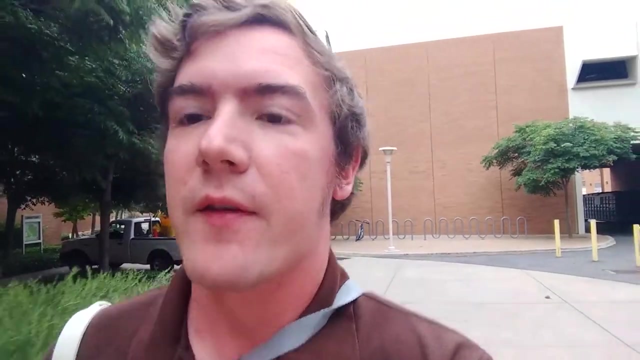 far, the combinations have been great here and, yeah, we're just going to see how this date goes. there's been a lot of good talks on botany, which, of course, is what I do. there have been talks on finds found on public lands and, of course, you know, yesterday I was in the the paleobiology database session, and so 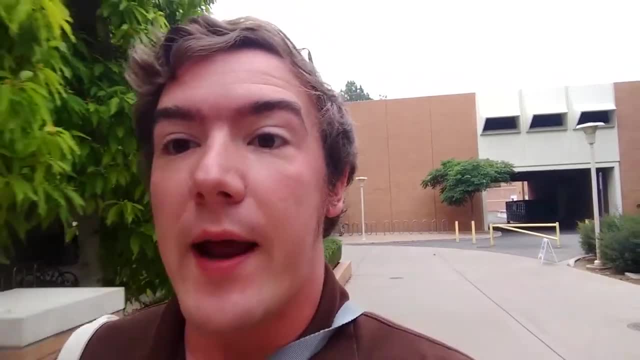 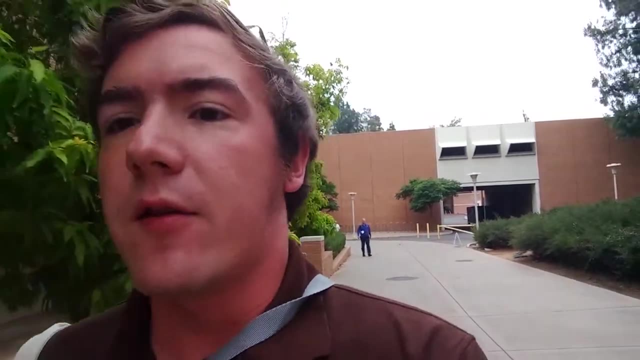 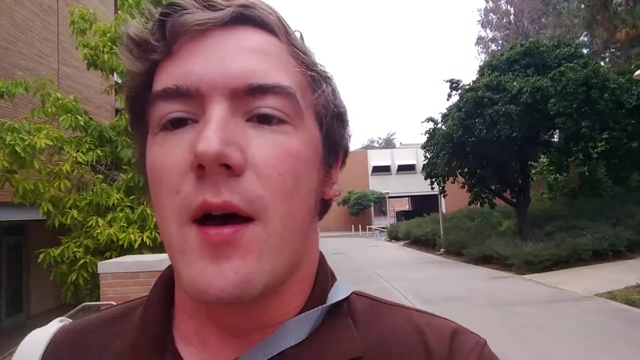 today. it's going to be on interactions between amateurs and professionals in paleontology. that's what I'm going to be speaking on, and this is one of a lot of people from fossil project are going to be speaking as well, so you'll probably see their faces appear throughout this video as 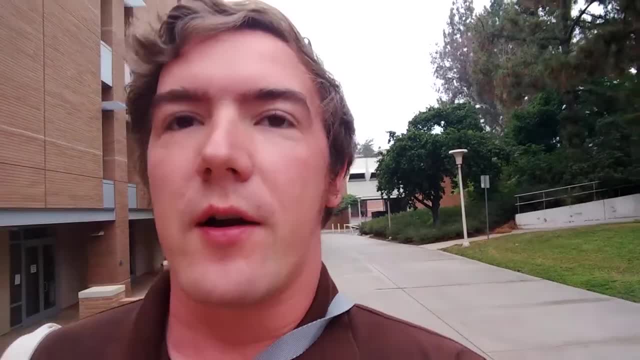 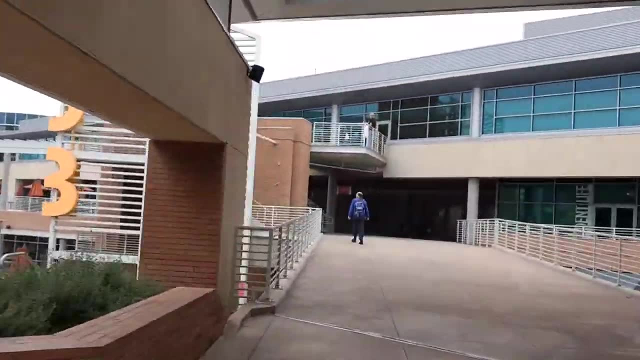 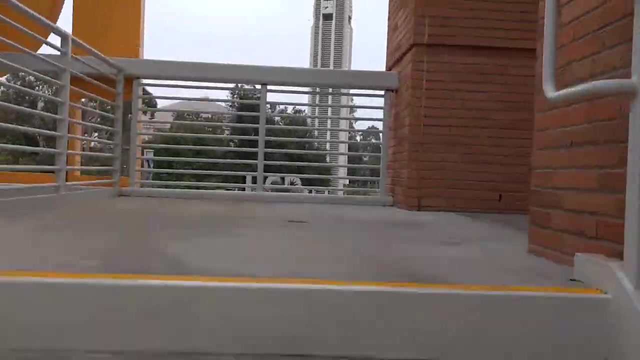 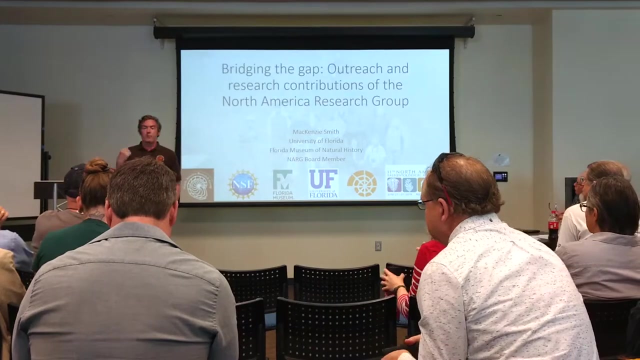 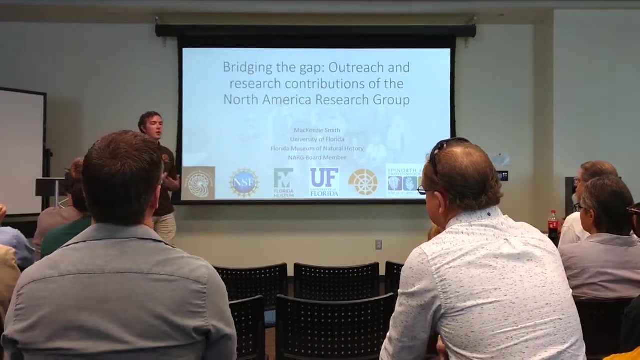 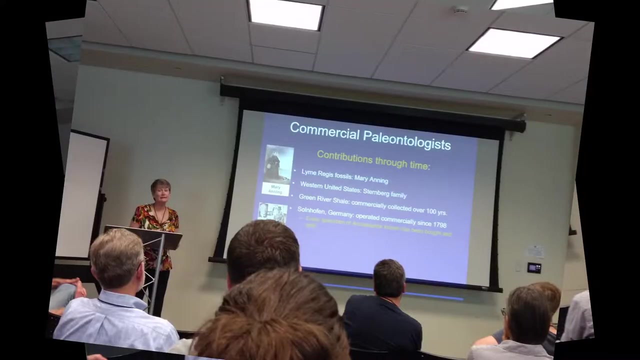 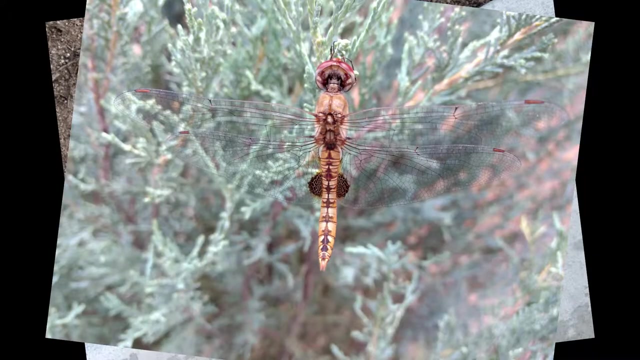 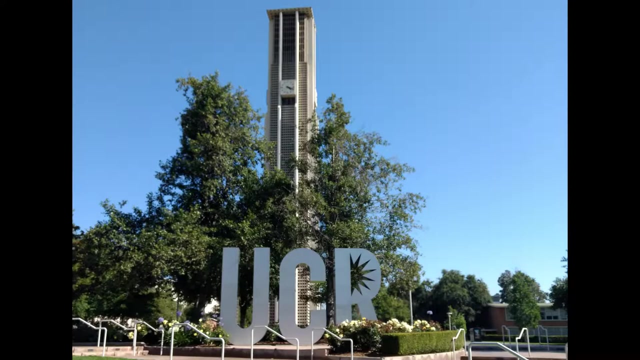 well, so let's continue on our way down to the talks. I will be talking about my home club, North America research group, also called GARD, music playing. so I'll yield the rest of my time to my colleagues and I will be talking about my home club, North America research group, also called GARD. 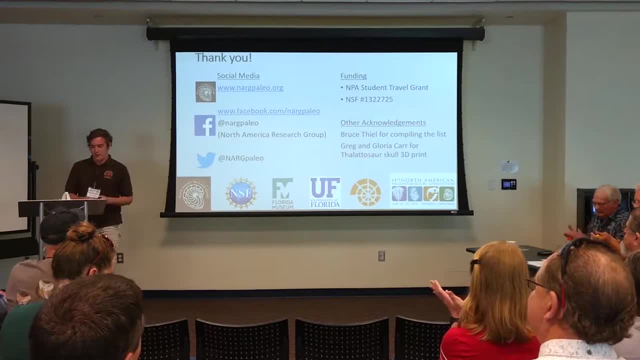 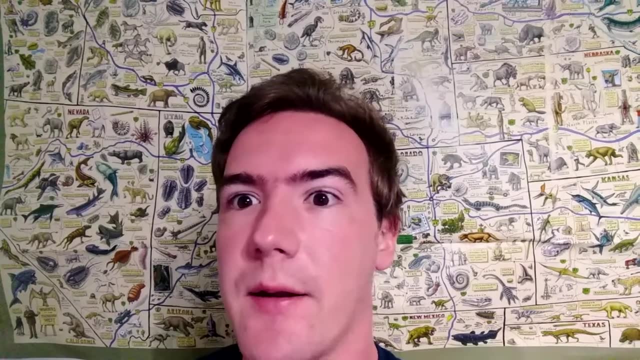 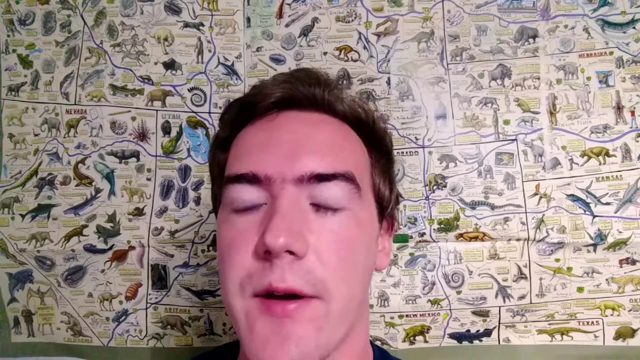 all right. so we're now back in Florida and I didn't have a chance to kind of go over like a little bit of a recap everything that happened, in sort of my final thoughts on NAPC, so I'll do that right now. the one thing I forgot to: 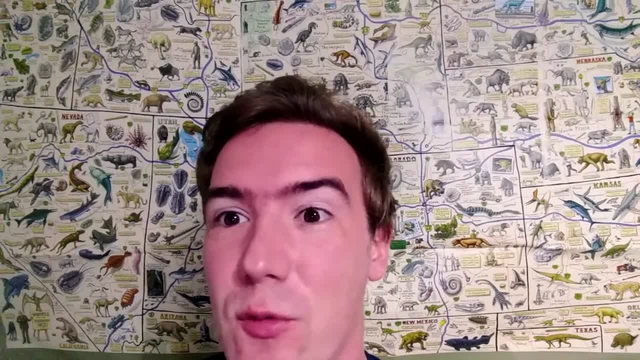 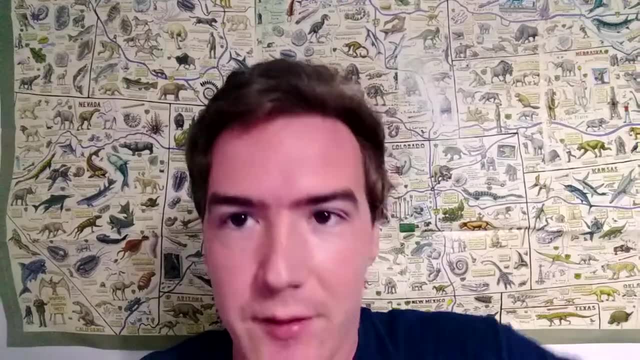 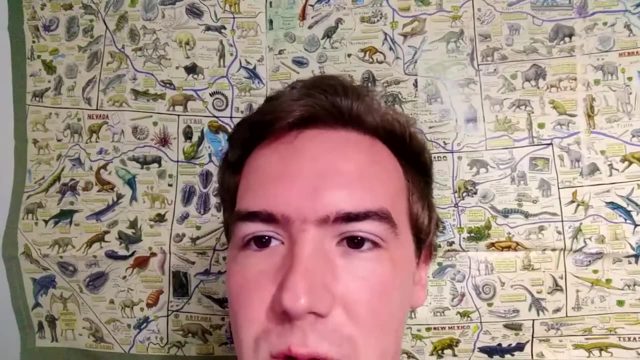 mention first was that when you check in you get a swag bag, so let's see if I can hold that up right here for the camera. it's nice little, nice little tote with the NAPC logo on it with all the pictures there and of course you know name tag that. 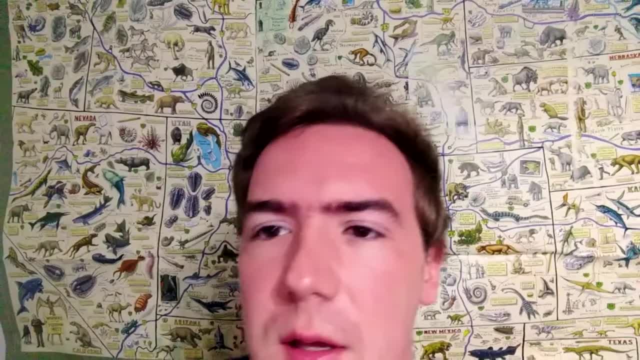 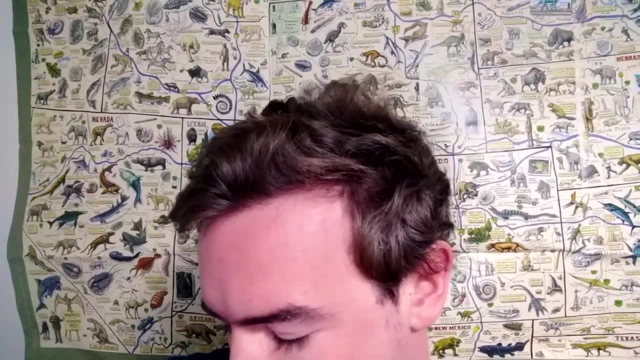 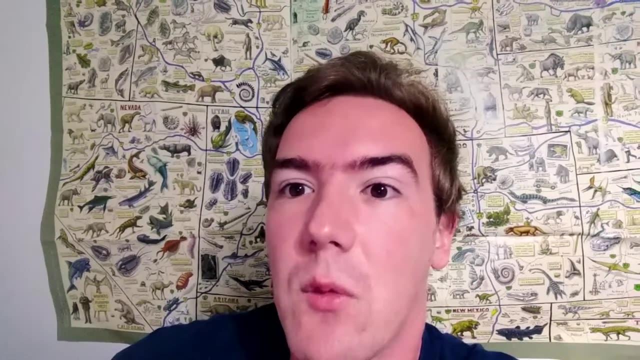 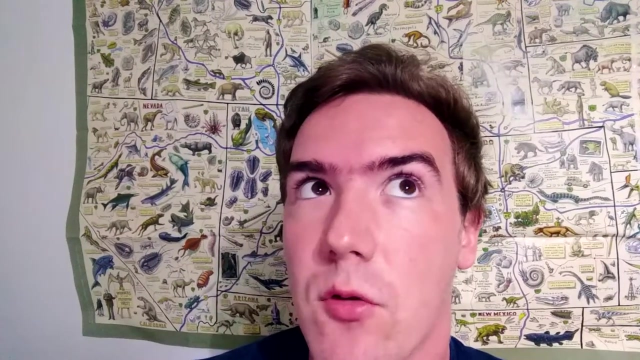 lets you get into the talks and also the meals and coffee. and you also get a water bottle. sadly, the logo rubbed off a little bit, but it's still, you know, pretty cool looking water bottle. in terms of the conference itself, I think it was great. this was easily my favorite academic conference that I've been to. 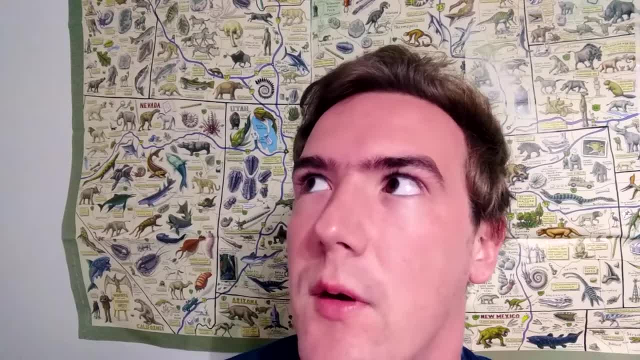 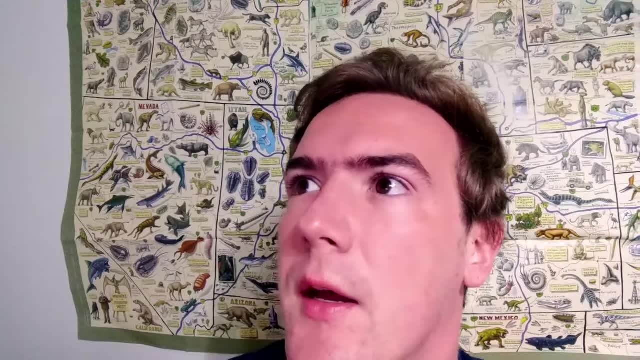 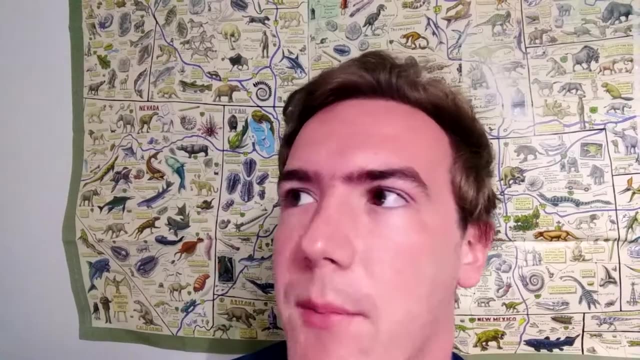 and I think there's a couple of reasons for that. so the first couple conferences I've been to, they were botany or geology conferences. one of the reasons, you know, I didn't particularly care for those is because I didn't. one reason was probably because I didn't know a lot of people there. and and two because I don't really consider. 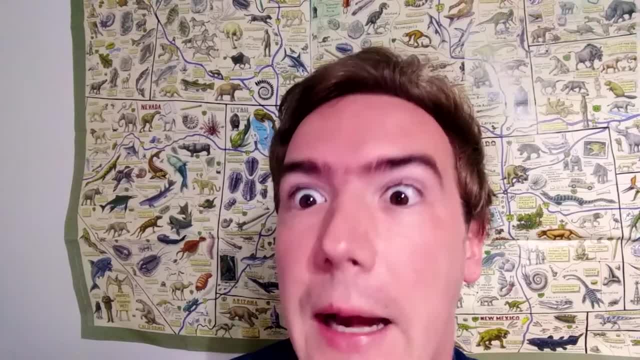 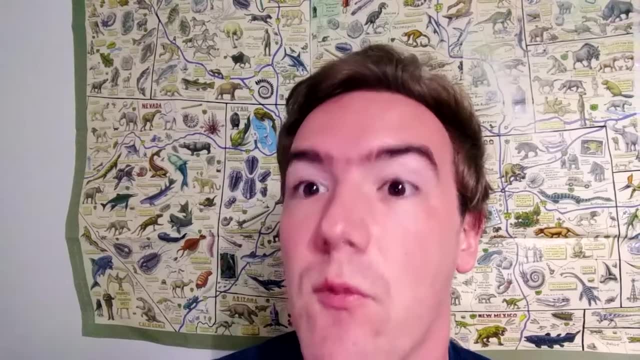 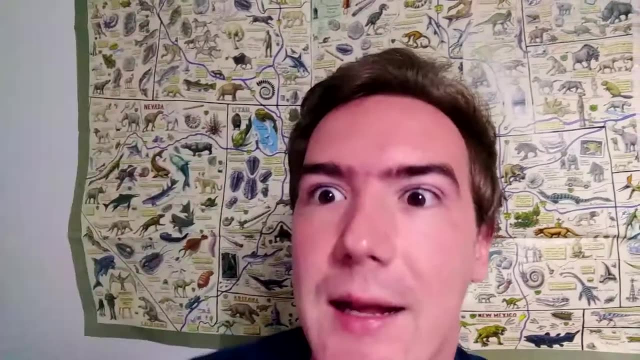 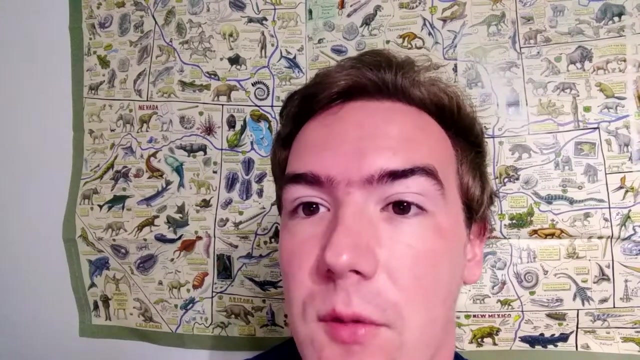 myself solely a geologist or solely like a botanist. I really do consider myself more of a paleontologist- and someone who does, even though I work with plants right now. I consider myself someone who's like interested in just anything, anything fossil, so that I think for 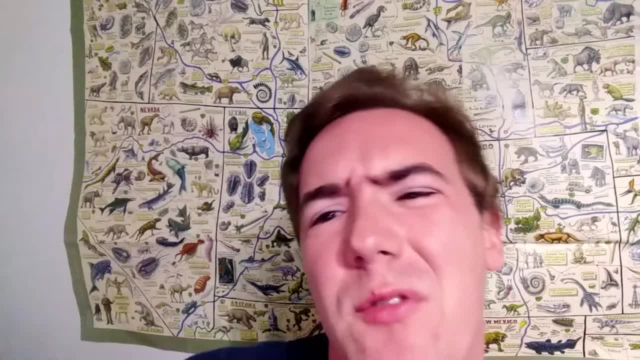 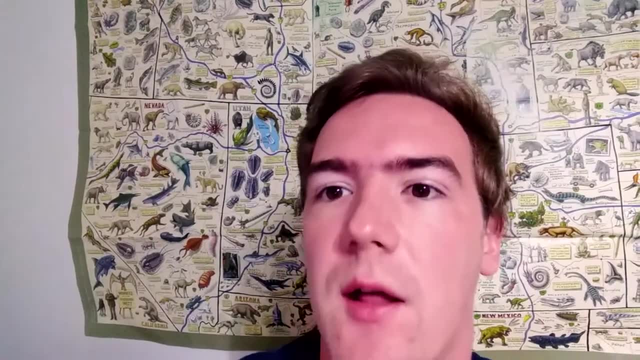 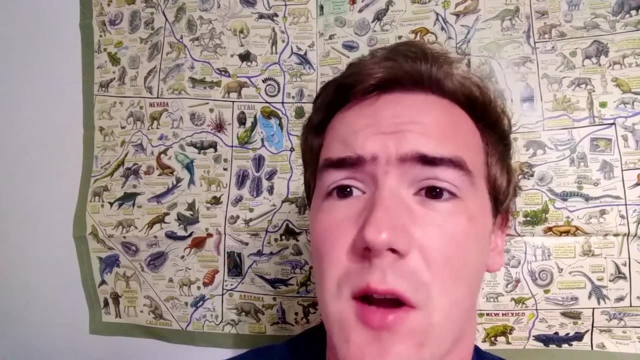 me this the overall theme, even though there's multiple themes within the within the conference. I think the overall arching of paleontology is a lot more interesting for me as an individual, and I think a lot of people also like this. this is a conference that only happens about once every four. 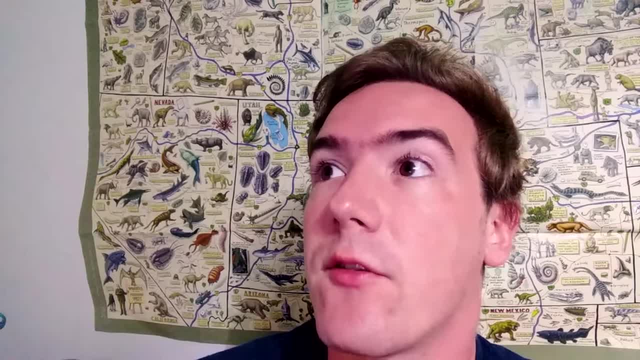 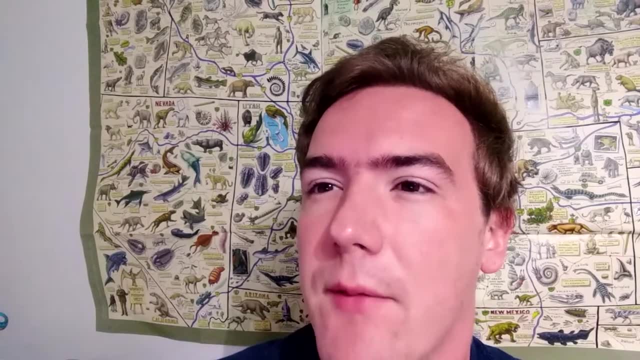 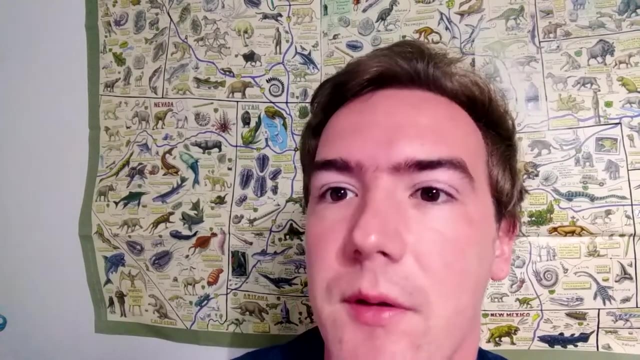 to five years, and so it's not as frequent as these other botanical or geological conferences, and so I think that kind of makes it a little more special in a way, but in ways I'd also like to have it more frequent in order to, you know, keep that sort of engagement. what else do I have to say? it sort of 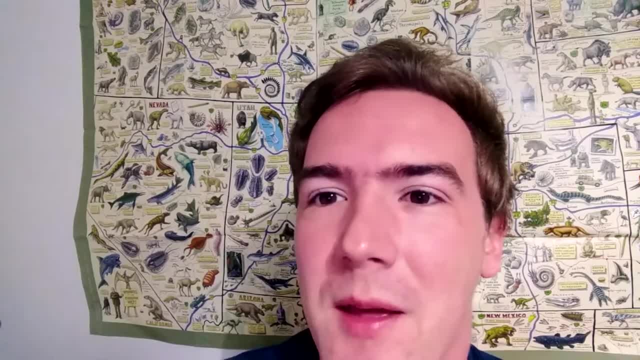 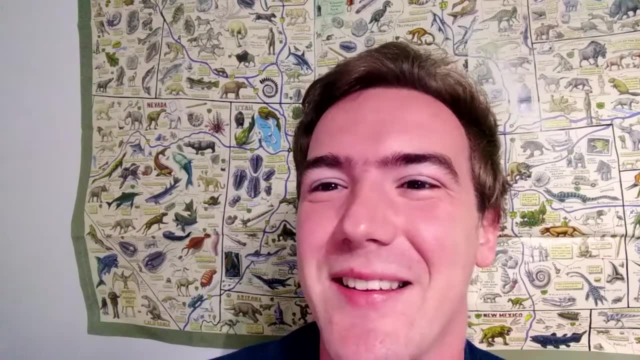 feels like a sporting event in a way that reminds me of being in a swim meet. you know, instead of you know waiting for your race, you're waiting for your talk and it would kind of be interesting to kind of do a parody of you know. it's sort of like you know the hype for the Olympics, but you